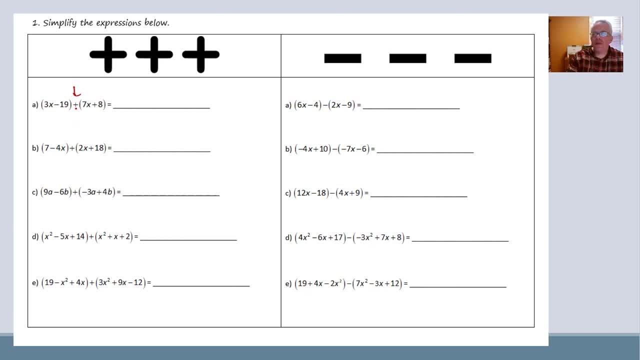 plus and minuses in these expressions. It's the one in the middle that tells us what the main event is. We're adding 3x minus 19 to 7x plus 8, so when we do this we combine like terms. We can combine the x's. 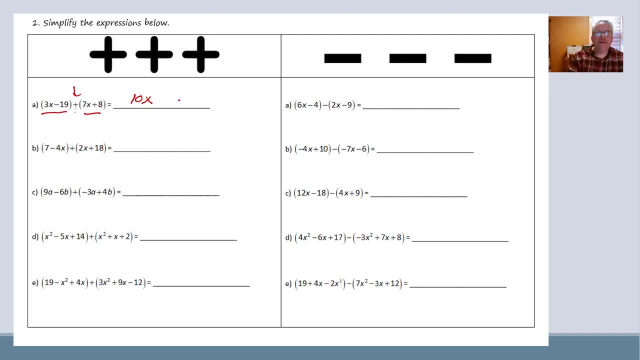 3x minus 19,. plus 7x is 10x Negative. 19 plus 8 is negative 11.. On this one they're not in the same order, but we can combine like terms: Negative 4x and 2x is negative 2x And we have a positive 7. 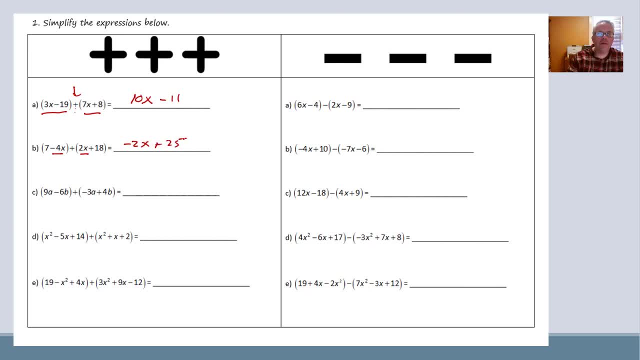 and a positive 18. That's 25.. We have A's and B's, No problem. We're just going to combine the like ones: 9a plus negative, 3a is 6a And a minus 6b plus 4b is minus 2b. We have two trinomials here. 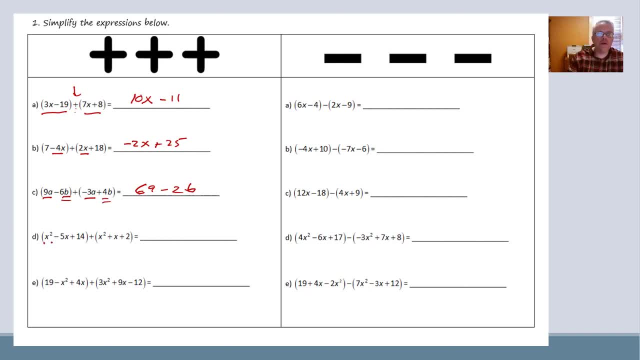 We have x squareds, x terms and constants, So I'm going to start with the x squareds: 1x squared plus. another one would be 2x squared Minus 5x plus 1x would be minus 4x. 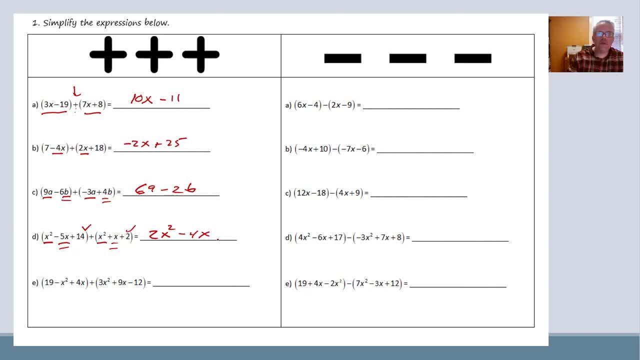 And we got the numbers left: 14 plus 2. That's going to be 16.. All right, This one's addition. again, We're doing the first trinomial plus the second one. This time the terms aren't in order. 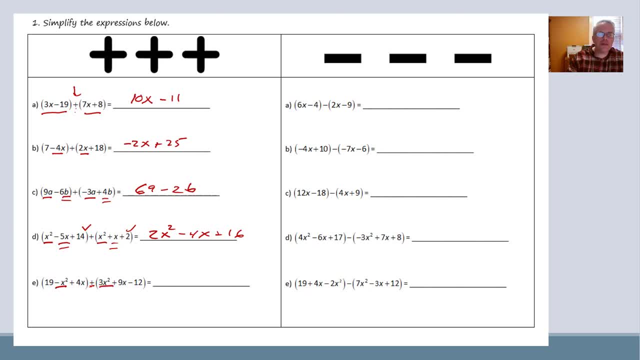 I'm going to still start with the x squared terms. There's minus x squared plus 3x squared is 2x squared. We have 19 and a minus 12. That's plus 7.. And finally, for x's, we got a 4x. there We can put that with a 9x plus 13x If we want to write it in standard form. 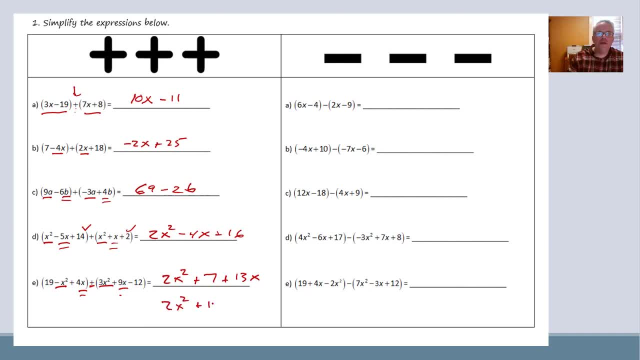 we put the quadratic term first, the linear term with exponent 1 next and then the constant next. But out of order is okay, All right. Now this is where things get a little trickier. This is subtraction, So we have subtraction in the middle. here We're doing this first binomial. 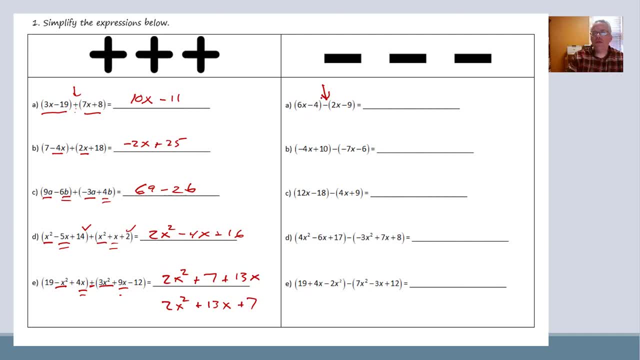 Minus the second binomial. So when I do this I take two steps. First I copy the first polynomial, Then I'm going to write what I get when I subtract the second one. We have minus 2x, So we're subtracting 2x. We are subtracting a negative 9.. That's the same as adding 9.. 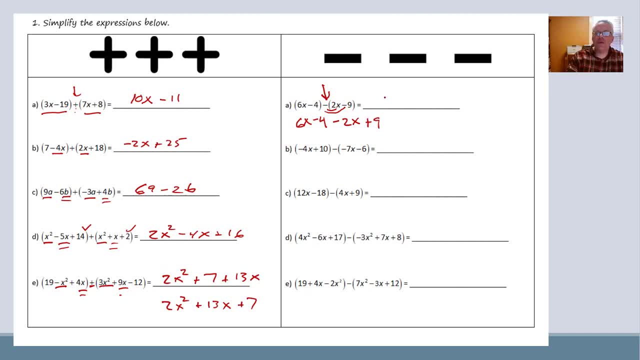 And now I can just add them, Combine like terms: 6x minus 2x is 4x And negative: 4 plus 9 is 5.. Okay, Here we go Rewrite Minus 4x plus 10.. We're subtracting a. 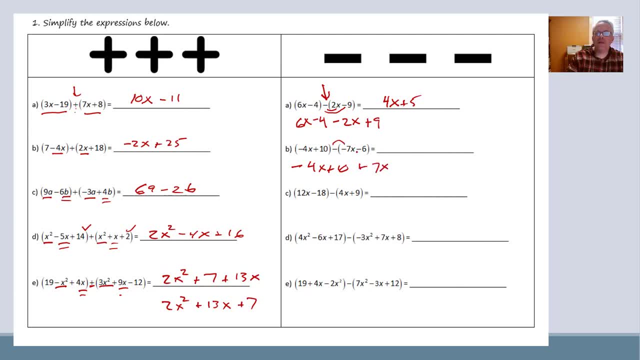 negative 7x, That's plus 7x. We're subtracting a negative 6. So that's plus 6.. Combine the terms And that's what you get. All right, First step: Rewrite The first polynomial. doesn't change. 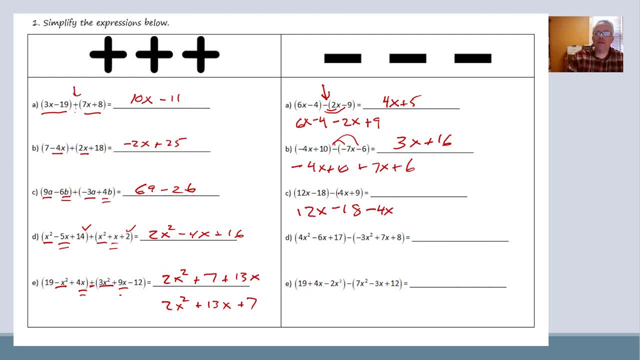 I'm subtracting the second one, So we're going to subtract 4x, And we're also subtracting positive 9.. So that's minus 9.. Combine them up, You get 8x minus 27.. All right, We're going to subtract. 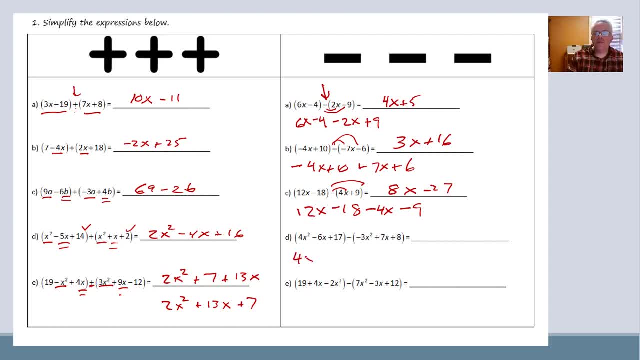 trinomials. No problem, Let's rewrite it though: 4x squared minus 6x plus 17.. Minus the negative: 3x squared is plus 3x squared, Minus the positive: 7x Minus 7x, And we're going to minus an 8.. So we have minus 8.. Combine like terms: 7x squared. 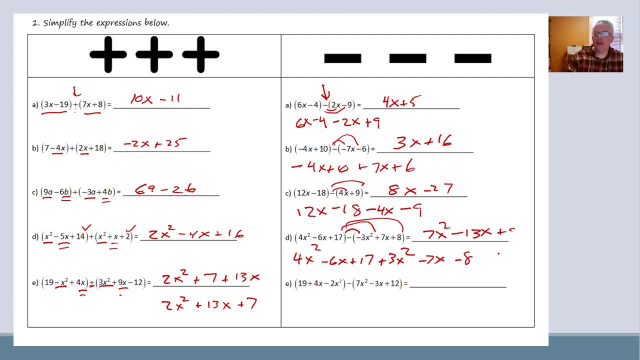 minus 13x plus 9.. Same thing here. The terms are in order, but that's okay. 19 plus 4x minus 2x squared Minus 7x squared Minus the minus 3x is plus 3x And minus the. 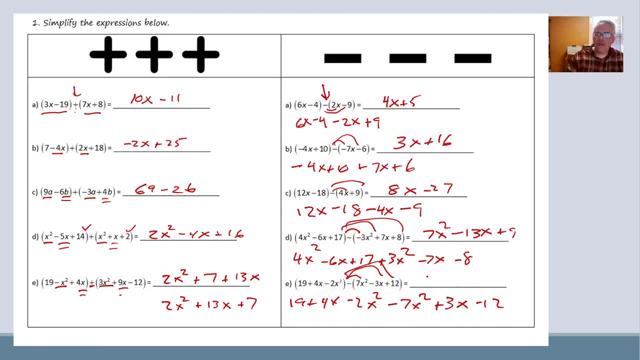 positive 12 is minus 12.. So 19 minus 12 is 7.. 4x plus 3x is 7x Minus 2x squared. minus 7x squared is minus 9x squared. All right, Look at that math. All right. Now just a. 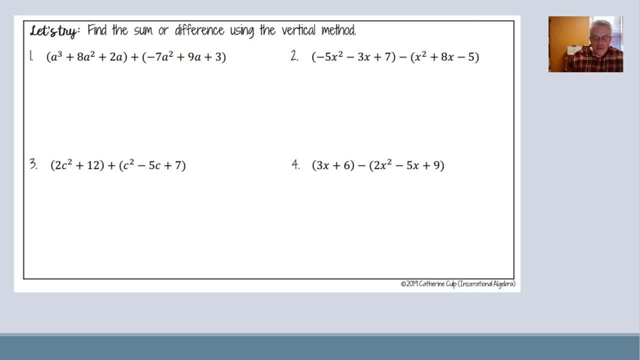 couple more practice problems and we're finished. Often they don't separate the addition and subtraction problems. You got to think: what kind of problem is this? Well, in this one we see that we're adding. Okay, So we'll just combine like terms. We. 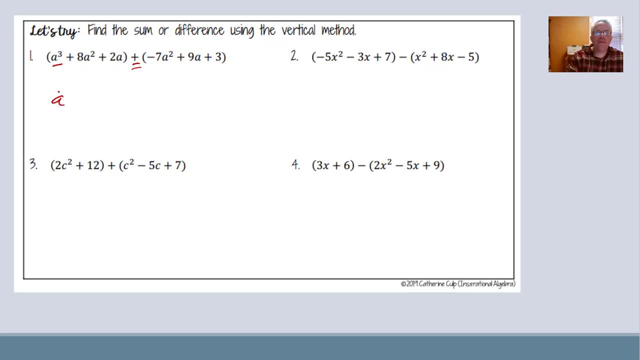 have a cubed. There are no other a cubed So I'll just copy it. We have an a squared and a minus 7a squared. I can combine those. I have a 2a and a 9a And the only constant. 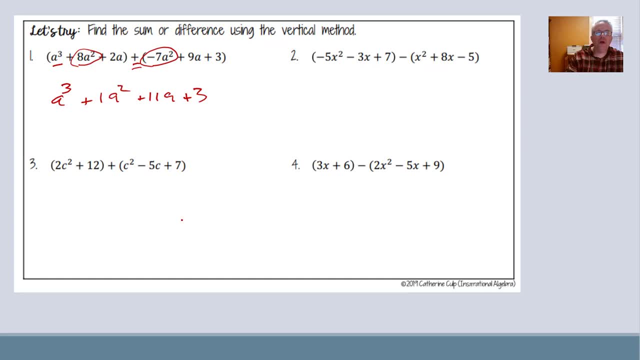 is 3.. I'm going to copy that down. All right, I'm going to work downwards. This one is addition also. So again, just combining like terms, We got 2c squared and 1c squared. We have a 12 and a 7. That's 19.. We have one. 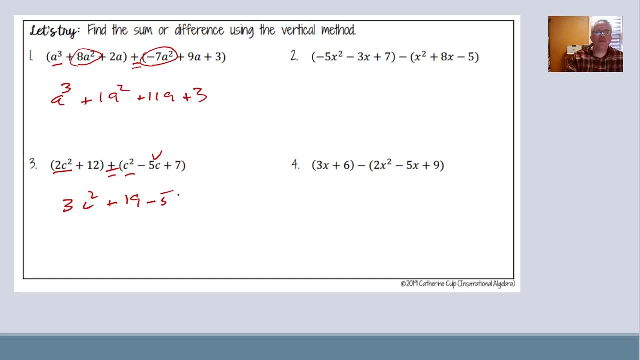 guy left over, There's minus 5c. There's nothing to combine with that, So I'm just going to write minus 5c, All right. And number 2, got to be careful, This is subtraction, So I'm. 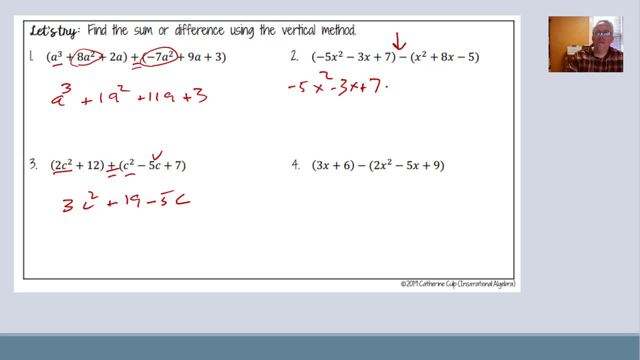 going to rewrite: Minus x squared minus 8x minus a negative 5 is plus 5.. And then just combine like terms: Same thing here. This is subtraction. Let's rewrite it: 3x plus 6 minus 2x squared minus.